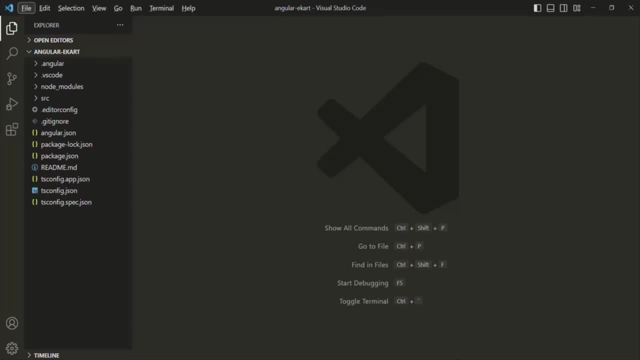 it generates a bunch of files and folders inside the project directory. As you can see, this Angular ECart is our project directory And in this project directory there are a bunch of folders and files that have been generated automatically when we used Angular CLI to 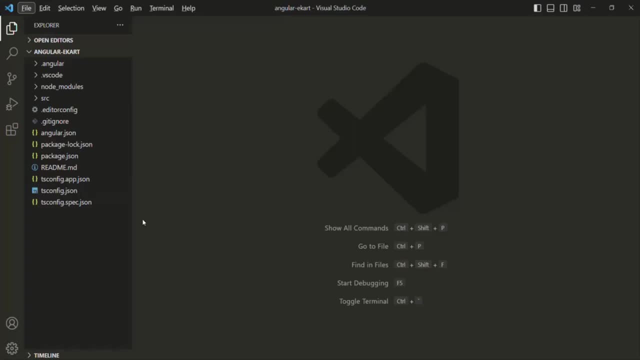 create a new Angular project And we created this new Angular project using ng new command. So when we use ng new command using Angular CLI, it creates a new project, It generates a bunch of files and folders which is required for that project, And each file and folder has its own. 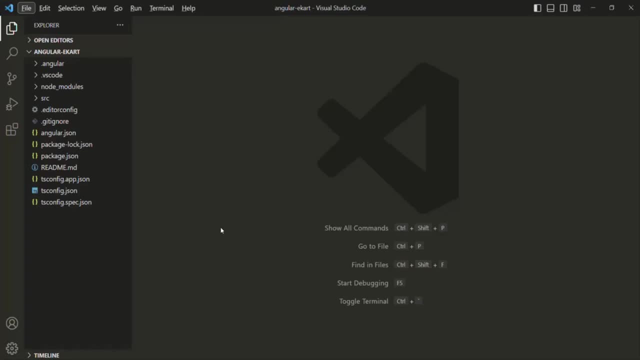 purpose. So let's see the use of some of the important files and folders of Angular project which you should know about, And let's start with this node modules folder. So this folder is where all the third-party libraries get stored, on which our application might depend on. So when we work on our Angular 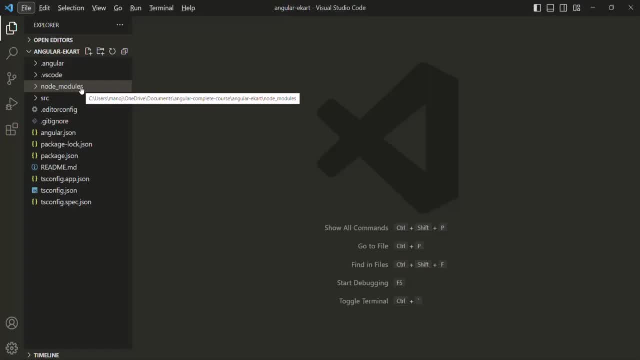 project we might need to use some third-party libraries and we might need to download those third-party libraries from npm. So whenever we will download those third-party libraries from npm, those libraries will get stored inside this node modules folder. Now this folder. 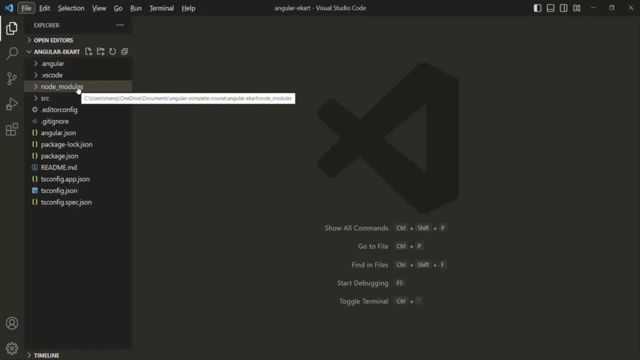 it is purely for development purposes And we don't deploy this folder in production server. Also, we don't check in this node modules folder in our repo. So let's say you're using git as your code repo And you want to share this. 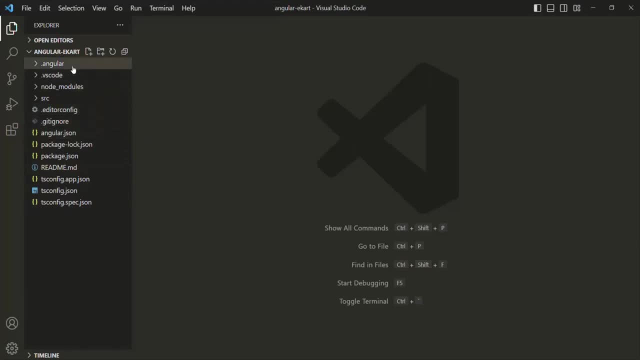 project code with your team members. So what you will do is you will push these files and folders in the git repo, And when you're going to push these files and folders to the git repo, at that time you will not push this node modules folder. As I said, it is purely for the development purpose. 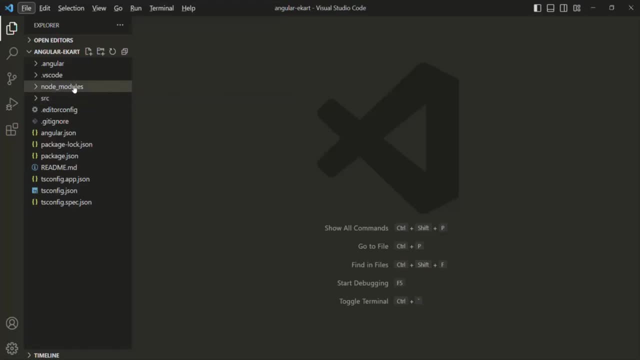 Now you might say Manoj, you said that in this node modules folder all the dependent libraries and packages will be stored. So if we don't push this node modules folder in the code repo or while deploying it in the production, then how the Angular application will work? Because the Angular 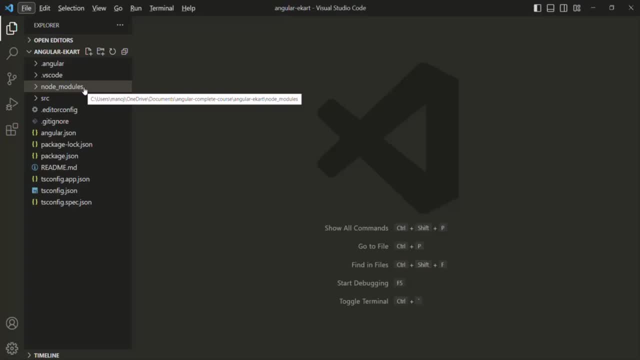 application is dependent on those third-party libraries. So how will this Angular application work? Well, what happens is so: for example, let me go ahead and let me delete this node modules folder. So now that node modules folder has been deleted, Now let's just assume that we have just checked. 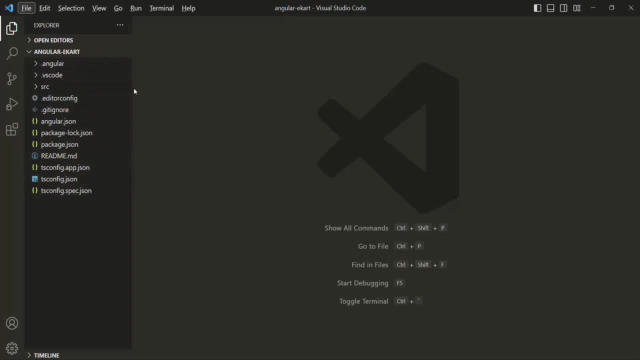 out this project code from the git repo or any other repo. So let's say my teammate has checked in this project code in the git repo or any other repo and I have just checked out this code from that repo And in there I don't have the node modules folder. 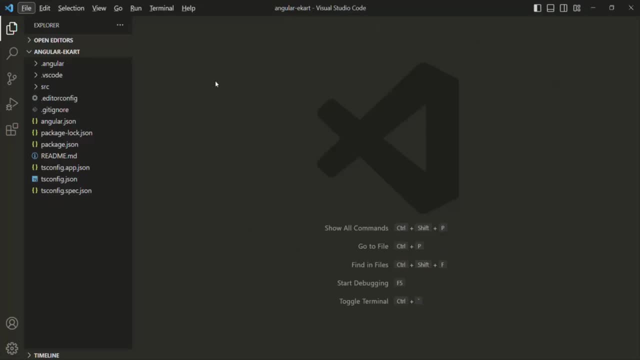 In that case, this Angular application is not going to work because it is dependent on some packages. the node modules folder is not there. that means those dependent packages are not available. this project is not going to work. so what do we do now? well, all we have to do now is we can open terminal. 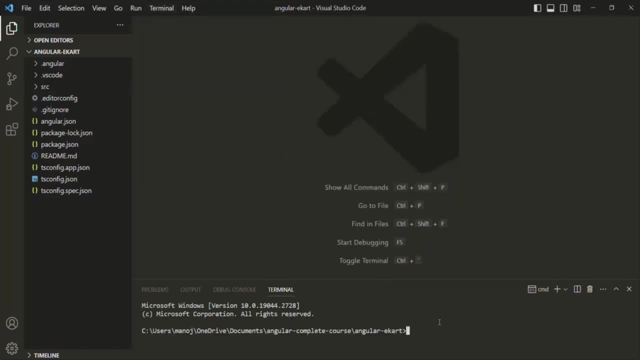 here. okay, or you can also use command prompt. let me clear the terminal here. and currently i am in the project folder. you see, this is my project folder path, and in the project folder path i just need to type an npm command, npm install, and then it is going to install all the dependent packages. 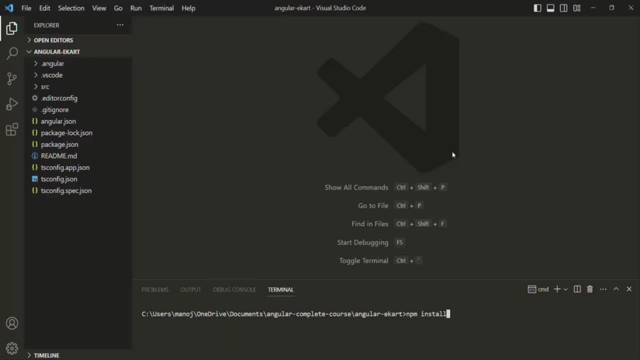 on which this angular project is dependent on, and it is again going to create that node modules folder and in that node modules folder we will have all our dependent packages. so if i go ahead and if i press enter, it is going to create the node modules folder again and in that node modules. 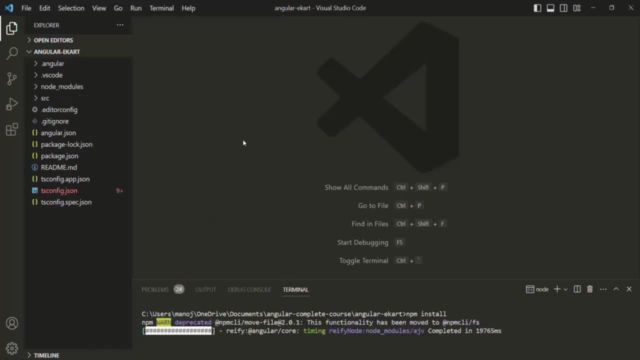 folder we will have all our dependent packages. so if i go ahead and if i press enter, it is going to packages. So you see, this node modules folder has been created and all the dependent packages and libraries are being downloaded and installed. All right, So all the packages have been installed. 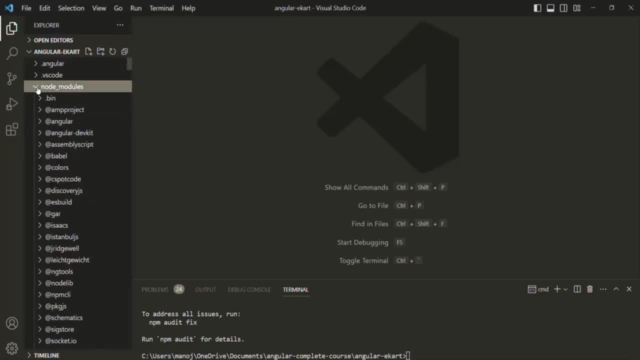 again. We have this node modules folder and in there we will have all our dependent packages. Okay, Now you might ask: all right, so we run this npm install command and it installed all the dependent packages for this Angular project. But how does it know on which packages this Angular 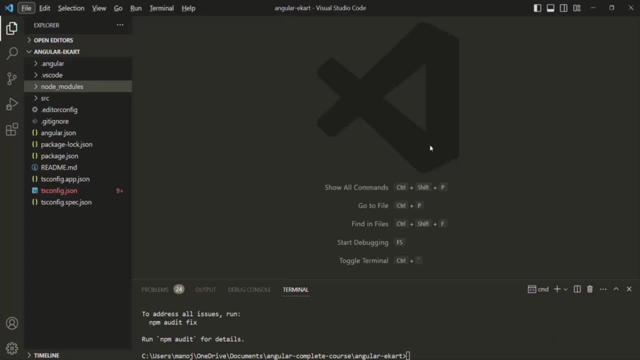 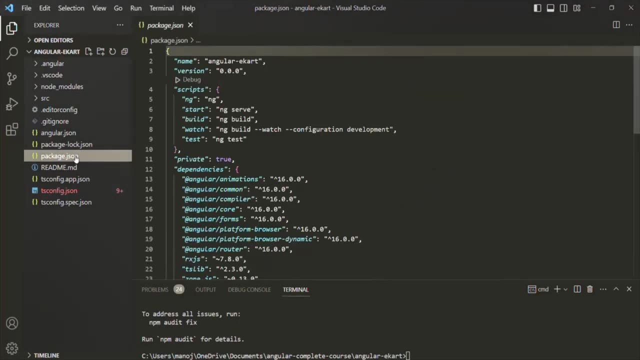 project is dependent on. That's where this packagejson file comes into picture. So let's talk about this packagejson file now. This packagejson file, it is one important file and this is a standard configuration file which every node project has. Now, this is an Angular. 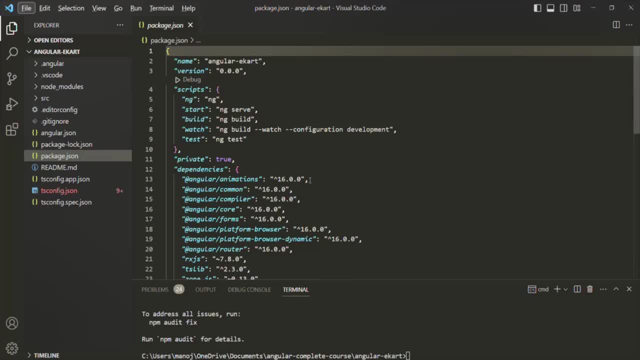 project, but here we are going to install packages from npm, Right? So every project which depends on npm will have this packagejson file And in this packagejson file you will have some project related configurations. For example, you can see the name of the project, the version of the project. Currently it is set to 0.0.0.. We can. 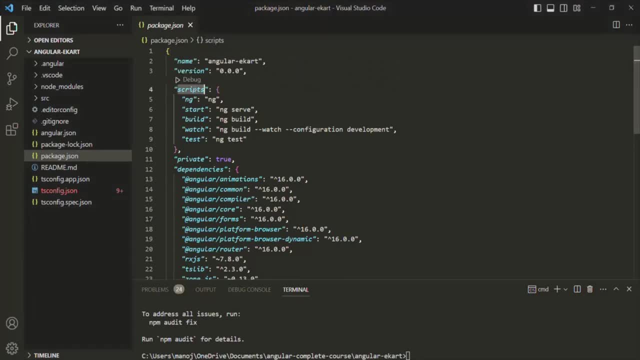 change this version. Then you can see the scripts which can be used in our Angular project. For example, in order to start this Angular project, we use this ng serve command. In order to build this Angular project. we use this ng serve command In order to build this Angular project. 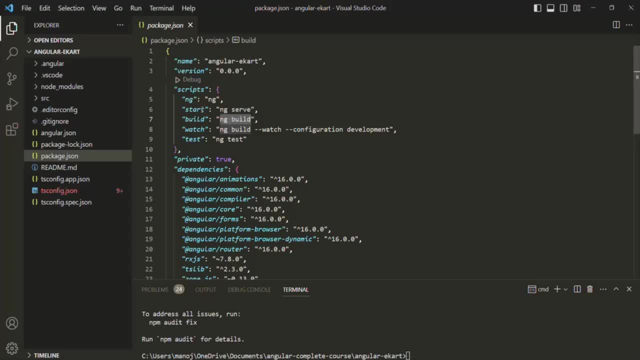 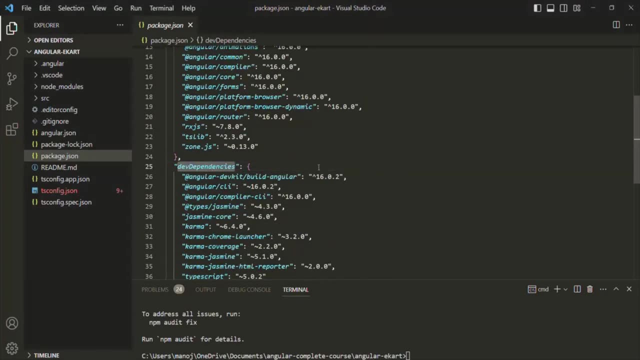 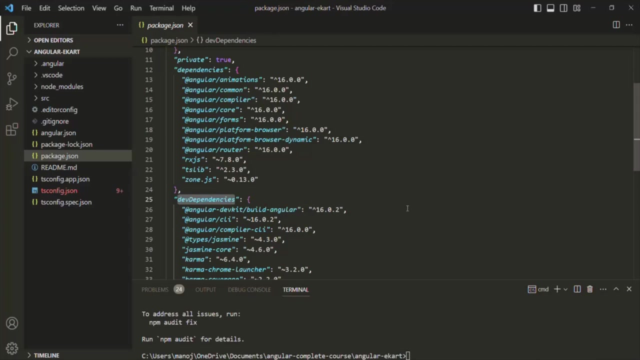 we can use this ng build command, Okay, And we have all other scripts. Then here we have two sections: dependencies and dev dependencies, And these two sections stores all the third party dependencies which this Angular project has. So, for example, this Angular project. 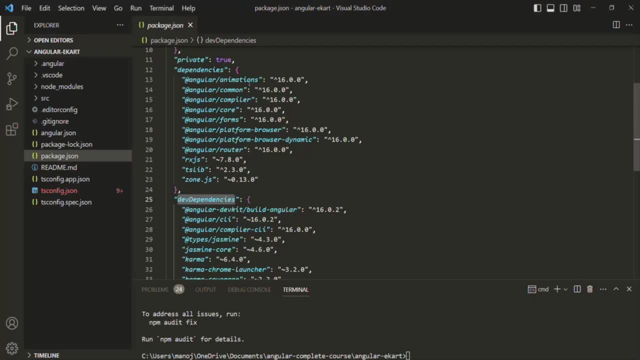 is dependent on these packages: This at Angular slash animation at Angular slash common, at Angular slash co. Let me actually show you that we are using this at Angular slash co in our project. So again, if I go to app component, if I open this app componentts file, 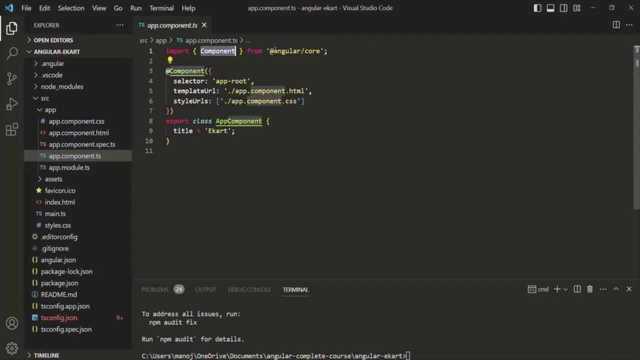 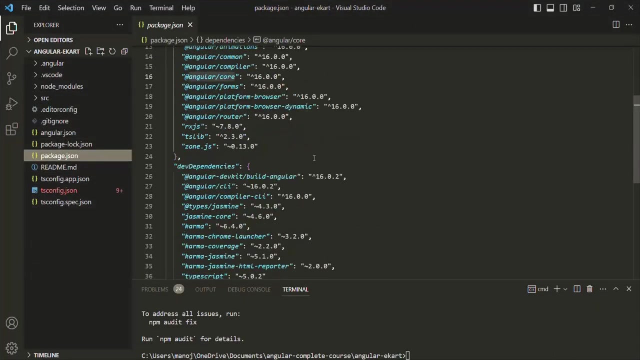 you see, here we are importing component from this Angular slash co package. Okay, So this Angular project is dependent on this package, So this packagejson file, it has all those informations, Okay, And we also have some dev dependencies. Basically, the difference between: 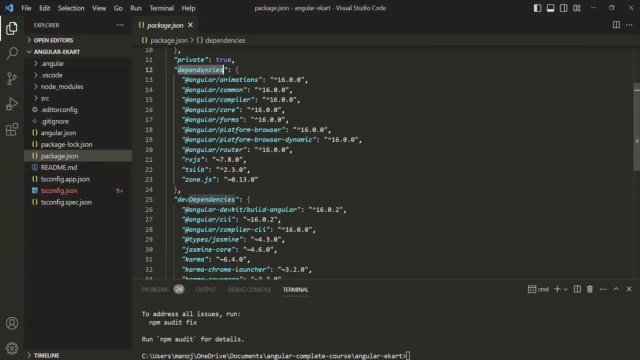 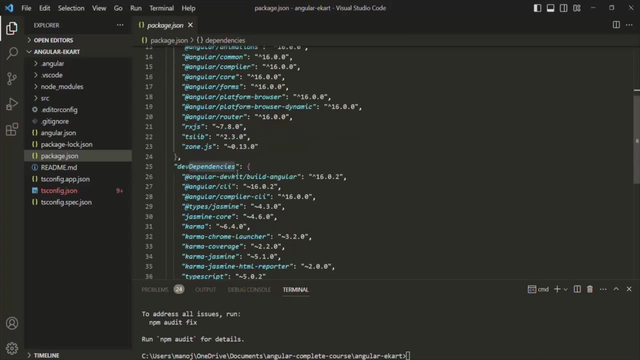 dependencies and dev dependencies is that in the dependencies we have some dependencies, So in the dependencies you will have the list of all those packages on which your project is directly dependent on, But in the dev dependencies you will have the list of all those packages. 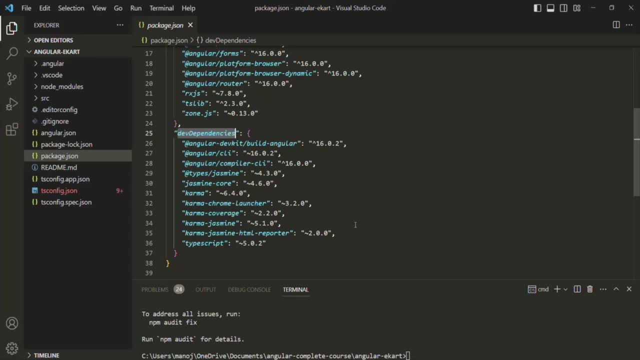 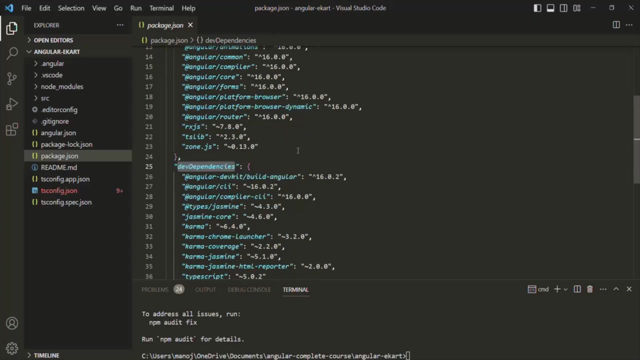 on which this Angular project is dependent on, while we are developing this Angular project. So these are all development dependencies. These are the tools which we might need when we are developing our Angular application. Okay, So here you can see the list of all the third party packages, all the third party. 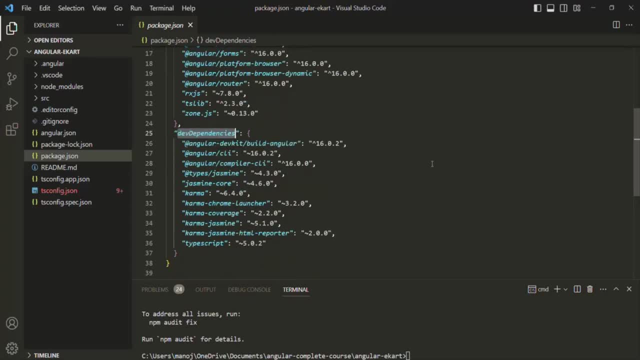 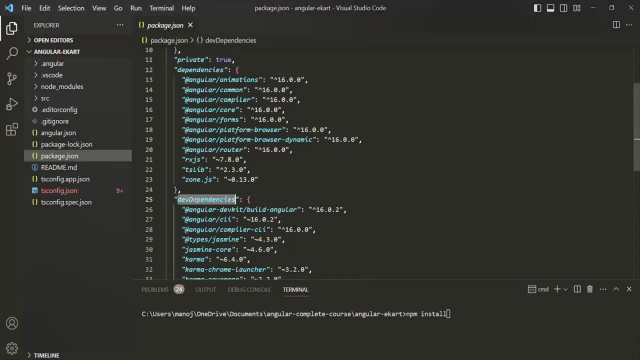 libraries project is dependent on. so when we type- let me clear the terminal again- when we type this npm install command, it is going to look inside this packagejson file, it will check for all the dependencies and all the dev dependencies and it is going to download and install all those. 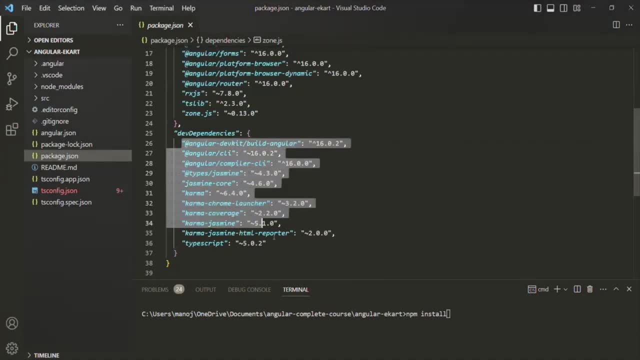 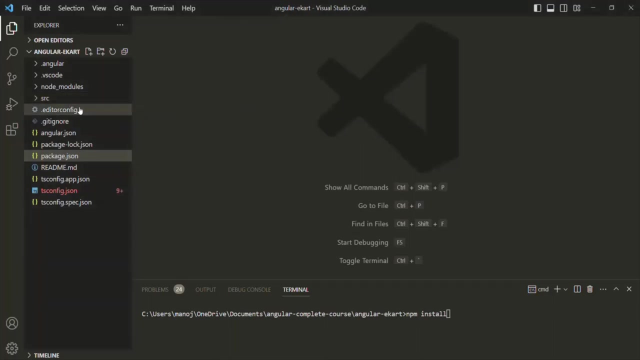 third-party packages. okay, so this is how npm install knows which packages to install and store inside this node modules folder. all right, then we have this source folder. we will talk about it later. let's go to this editor config file here. so this file. here it is basically used. 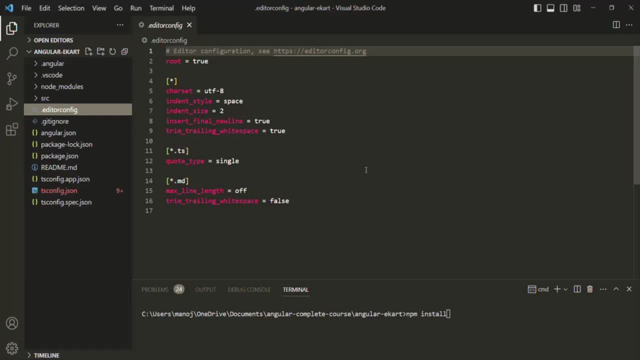 to set up the team environment. so in a real project many developers may work on a single project and each developer may follow different coding standards to declare variables, classes, style, size of each character, length, etc. but in the npm install command it will check for all the dependencies and all the dependencies. 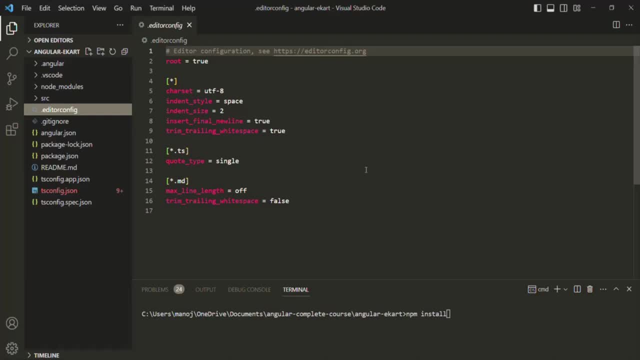 we need to merge the code of each developer to produce the final product right, and at that time it may produce some error or messy code, as each developer is having different coding standards. now, in order to solve this problem, this edit config file is used where the standard rules. 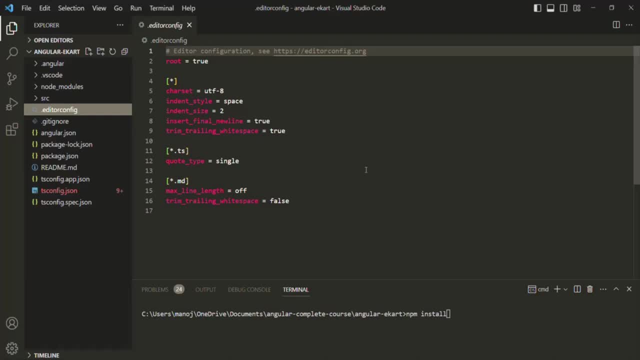 are defined, which needs to be followed by the developers in the teamwork, and, moreover, the developers do not have access to this file and only the manager or the team lead, who defines the rules, can only have access to this file. so, in order to solve this problem, we need to 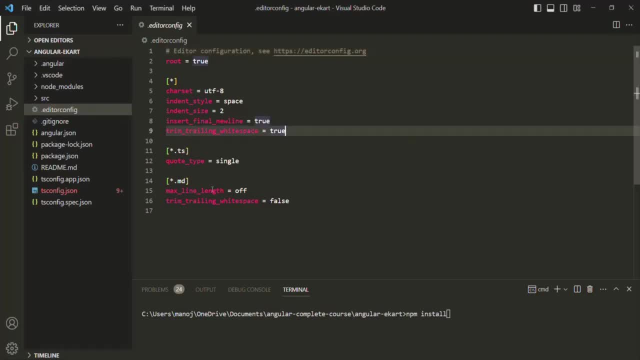 define the rules, and in this file you can see all those rules. you can define your own rules for the coding standard as well. now, while developing the angular application, we as a developer do not have to worry about this editor config file. it is the responsibility of the manager or the team lead, who 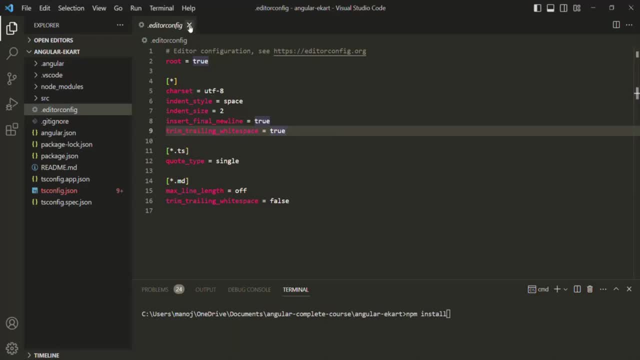 will define these coding rules. okay, let's close this file as well. and then we have this git igno file. so let's say your team is using git as the code repo. now, when you are checking in your code to the git repo, you might not want to check in all the files and folders in the git repo. 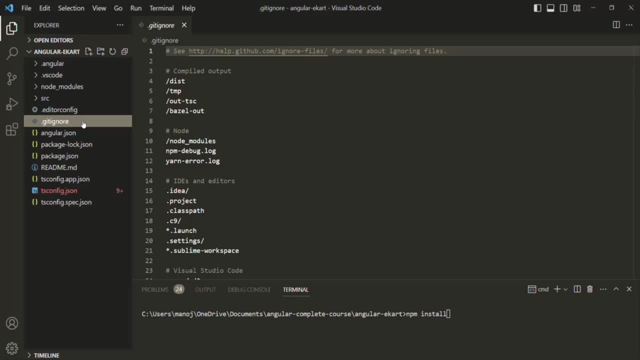 right. so in this file you can specify the files and folders which you want to exclude from your git repository. if you have these folders in your angular project while checking in in the git repo, so these folders will be ignored. then you can see we are also ignoring this node. modules folder. 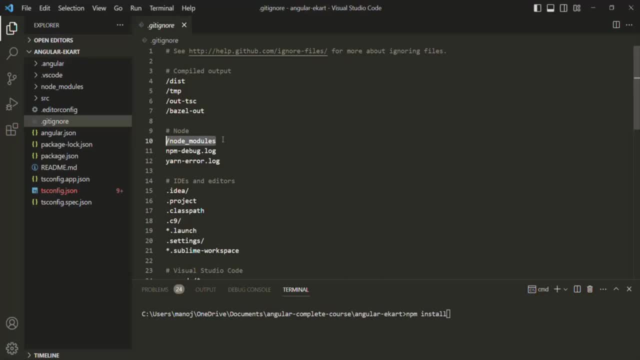 as i mentioned, we are not going to check in the node modules folder in the repo. then if you have these files in your project, these will also get ignored and you can specify all the folders and files which you want to ignore, which you don't want to check, into git repo. so let's say, in my angular project i have created a new folder. 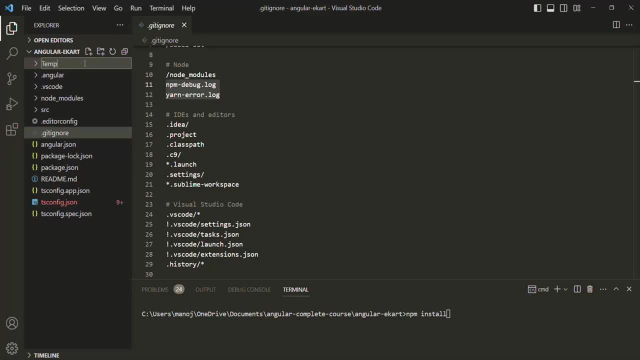 i will call it maybe temp, and in this step folder i am going to keep all the files which is not required for checking in. for example, in this stem file i am going to keep some notes or maybe the design document or something like that, and i will also keep the default files, which is in the git repository, so i'll only need to check. 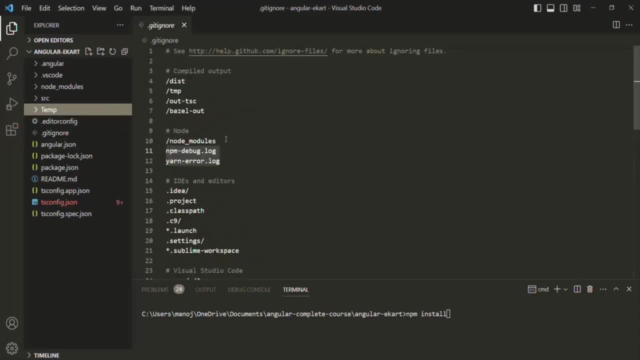 in those files in the git repo. so i want to ignore this file to be checked in into the git repo. for that i can simply go ahead and i can include that folder here so i can say slash, temp. so this folder will be ignored and all the files which we have inside this folder that will also get ignored. it. 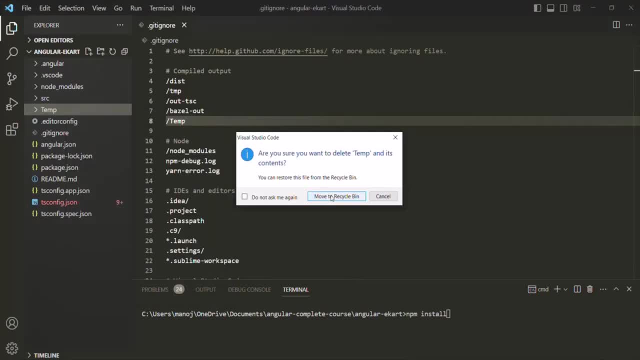 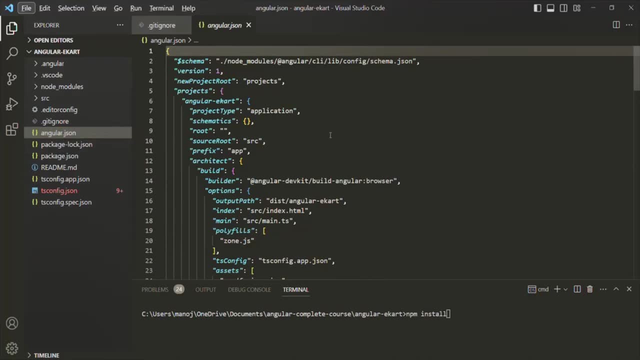 will not get checked in in the git repo. okay, i hope it's clear. let me go ahead and let me delete this folder. have this angularjson file now, this angularjson file. it is one of the most important files and it contains all the configuration of your angular project. so here you can see the project related. 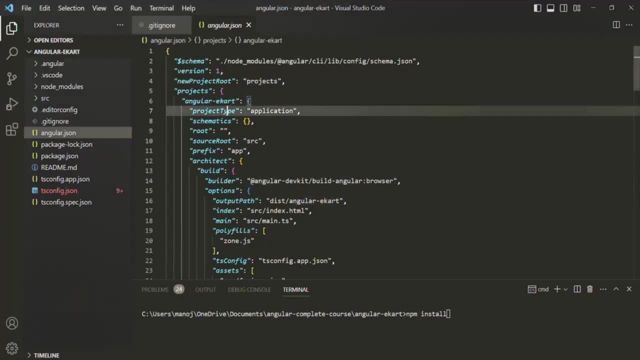 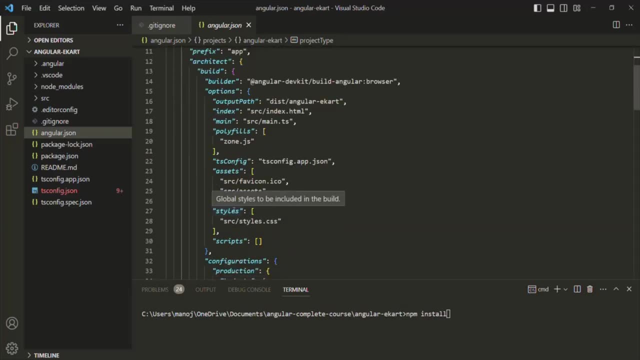 configuration. the project name is angular cart. project type: it is an application. then we have all other configurations. for example, what are the style sheets we are going to use and where to find it? so we are going to find the stylecss in the source folder. then what are the scripts we want? 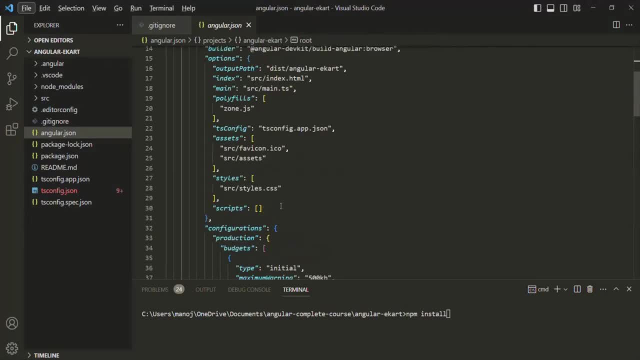 to use. we can specify it here inside this array. here you can also see which file should be loaded when the angular runs for the first time. in this case it is indexhtml file which is present in the source folder. what is the main entry point for the angular application? in this case it is maints so. 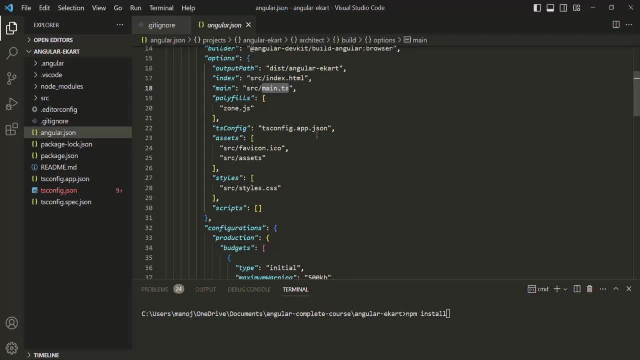 all these angular related configuration you will find inside this angularjson file. now we are going to talk more about this angularjson file in our next lecture. for now, this should be. it. just keep in mind that this angularjson file is the most important file here and it contains all the configuration related to. 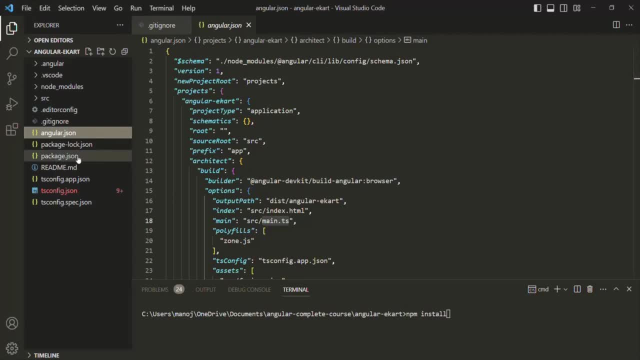 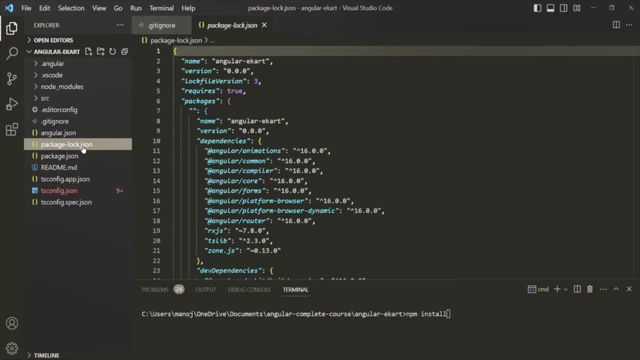 our angular project. now we already talked about this packagejson file. we also have something called as package logjson. now this package logjson file: it records the exact version of every installed dependency, including its sub dependencies and their versions. the purpose of packagelogjson is that it ensures that the same dependencies are installed consistently across. 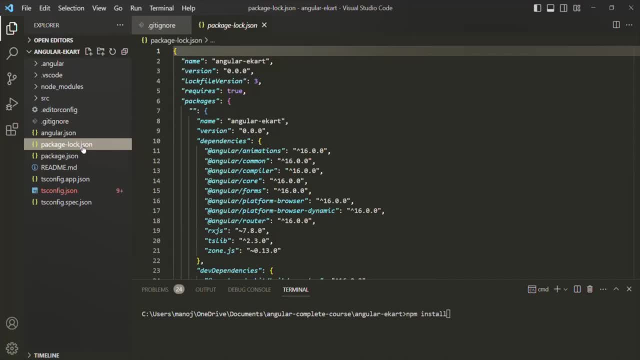 different environment. for example, we might be deploying our angular application in development environment, production environment, integration environment. so in all these environments the same version of all the dependencies gets installed. this job is taken care by this package logjson file. then we have this readme file. we don't need to worry about this file. let's close this one. 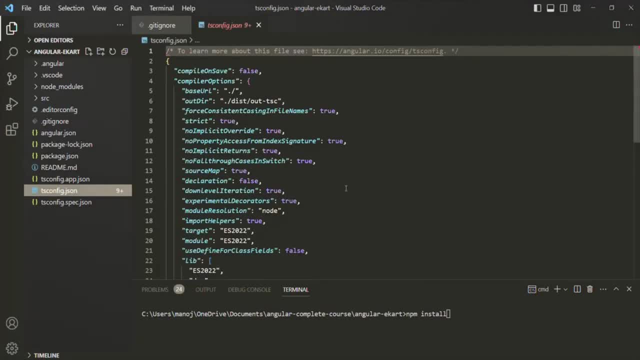 then another important file which we have is this tsconfigjson file. this is the file which is used to compile your javascript code, and it contains a bunch of settings for your typescript compiler and typescript compiler. look at these settings and, based on these settings, it is going to compile your typescript code into javascript. 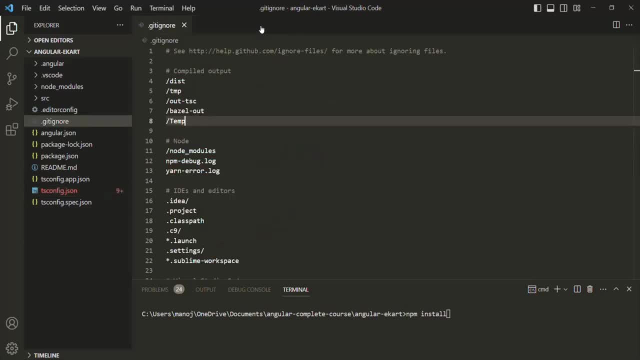 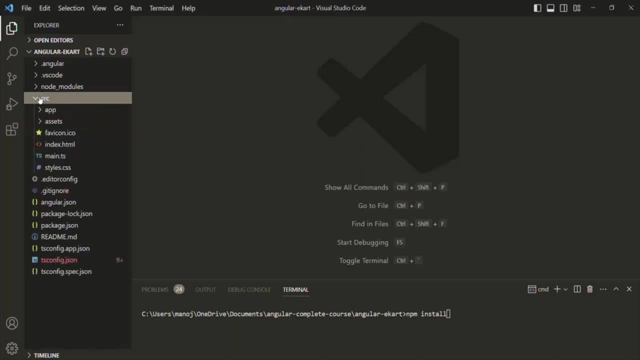 that the browsers can understand, but for most of the part, we don't have to worry about this tsconfig file. okay, let's close this one. let's also close this gitignore. and now let's talk about this source folder. so this source folder is the most important folder and you, as a developer. 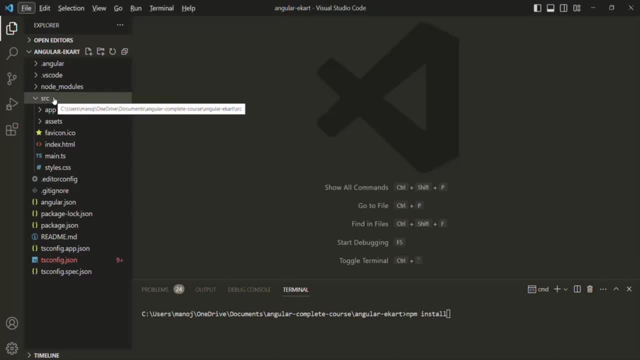 need to have a lot of files and folders inside this source folder. it is this source folder in which we put all our application source code. so every component, service class modules, everything we need in order to create an angular application that goes inside this source folder. now, whenever. 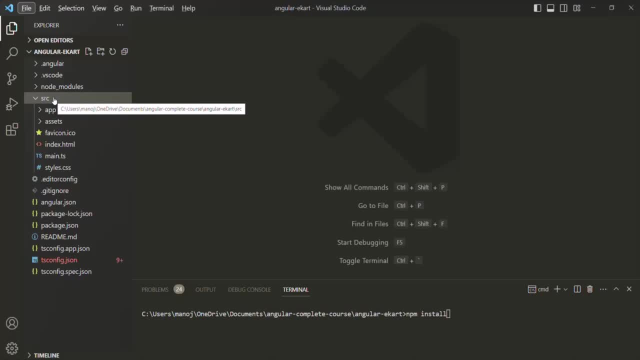 we create an angular project. by default, angular framework creates a lot of files and folders within this source folder and you can see those folders and files here. so first of all we have this app folder. this is the application folder. whenever you want to create any component, service or module, you need to create it within this app. 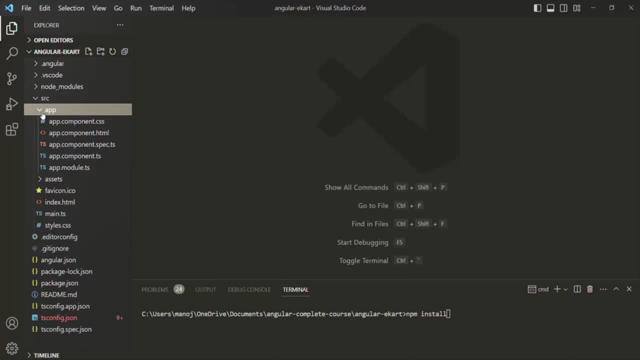 folder. okay, so just remember that in an angular project we can have multiple applications and by default we get one application and that application is available inside this app folder and inside this app folder, by default, we have one app component. so these four files together they create a component and we are calling it as app component. 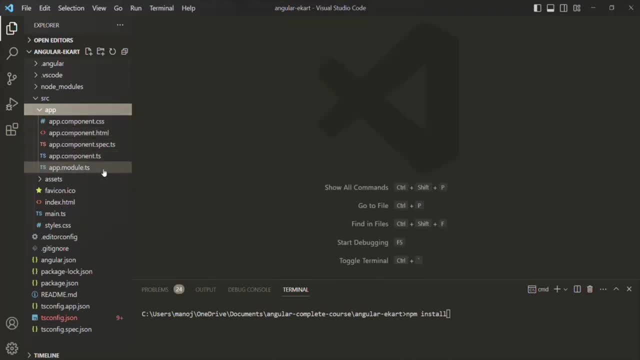 and then we also have this app modulets file. so again, remember that every application which we create in an angular project, every application will have at least one module file. okay, so every angular application must have at least one component and one module. in this case, for this application, we have one component, so these four files together will create one component. 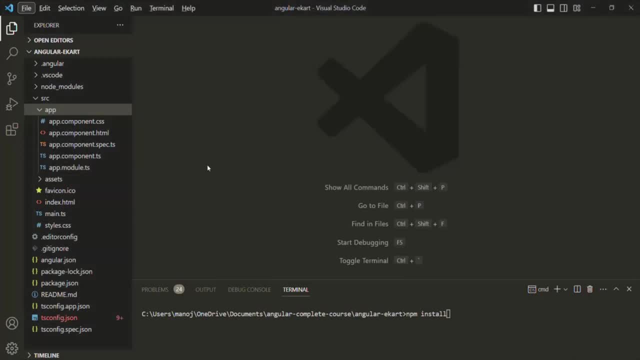 and we have one module now. we are going to talk about module file and we are going to talk about how to transfer modules and components in great detail in our coming lectures, so we will not worry about that right now. i will close this app folder. then we have this assets folder now in this. 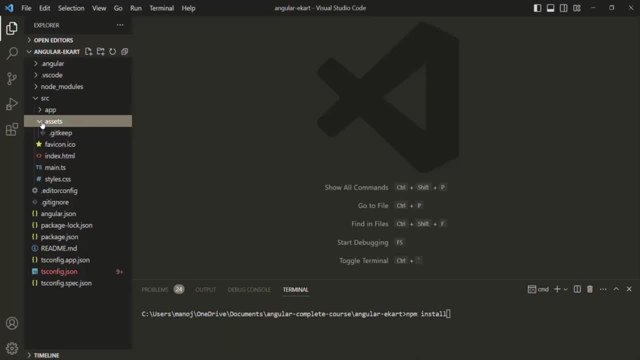 assets folder. we store all our static assets, for example, images, icons, text files, etc. and whatever we store inside this assets folder that will be public and that can be accessed. for example, let me go ahead and let me add an image inside this assets folder. I'll come back in a minute. 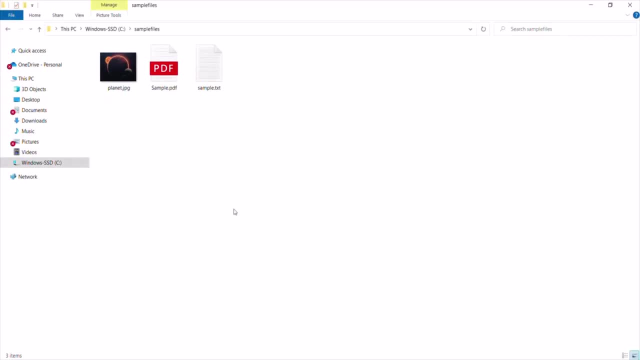 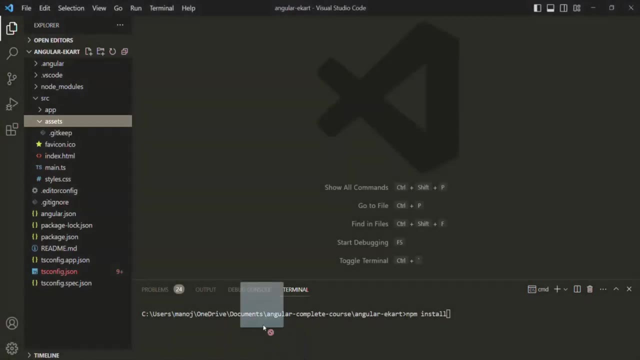 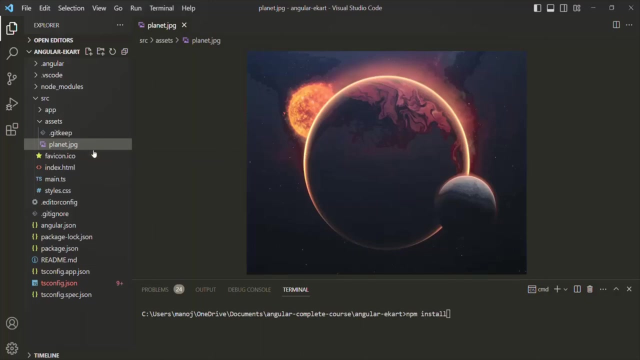 folder. for that, let me go to this folder. here I have this sample files folder and in there I have one image. I'll just drag this image, I'll open vs code and I will put this image inside this assets folder. okay, so here we have this planetjpg file. now let's try to access this. 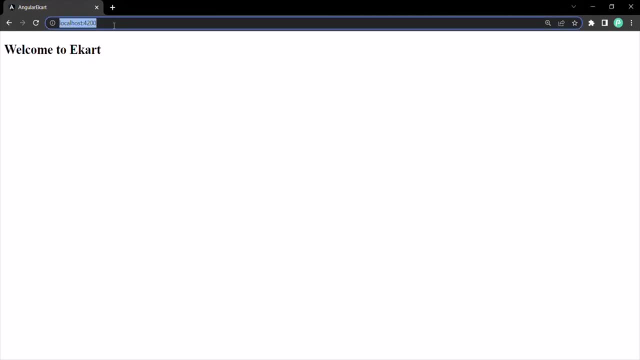 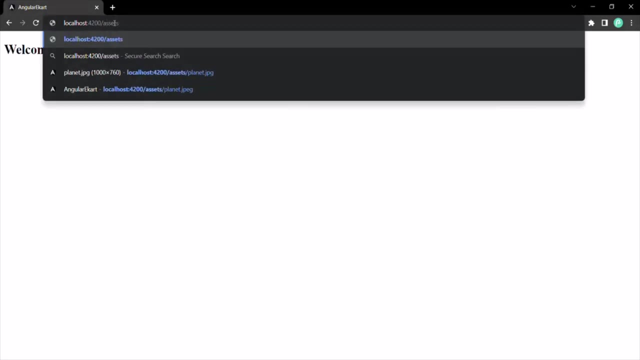 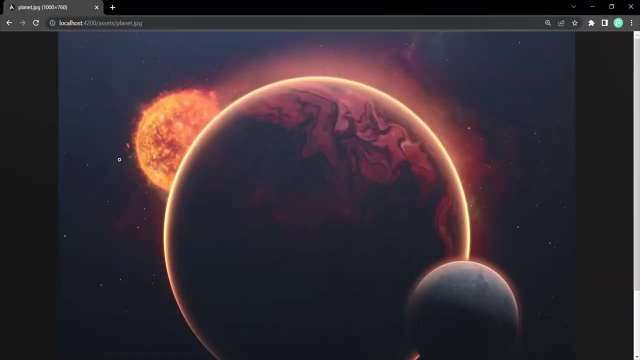 file from the browser. let me go to the browser and there let's type root URL, which is this: localhost, colon 4200. then we have the assets folder and in there we have planetjpg. if I press enter, you see that image has been rendered here. so whatever file and folder you will place inside this assets, 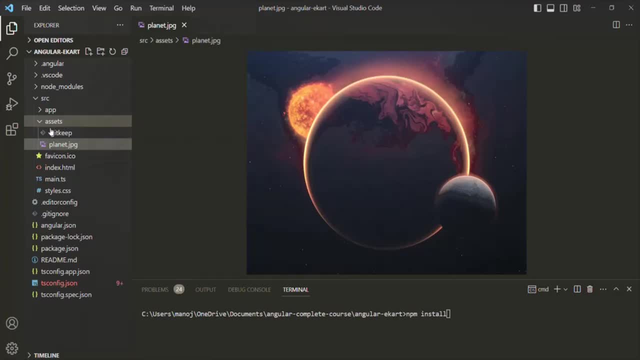 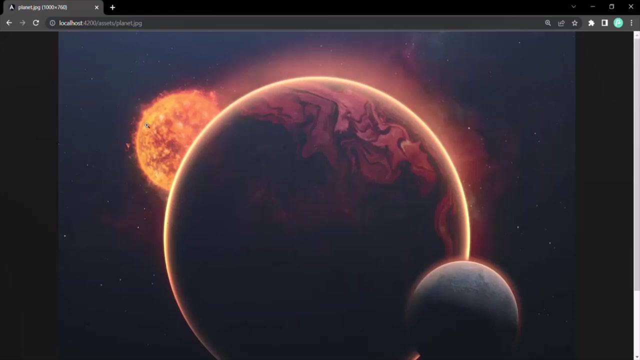 folder that will be publicly accessible. you can even put it inside a folder. so inside this assets folder, let me go ahead and let me create a new folder. I will call it images and in that images, let me go ahead and let me put this planetjpg. okay. so now, if I go to the browser, I will have to specify that path. so in the assets folder, 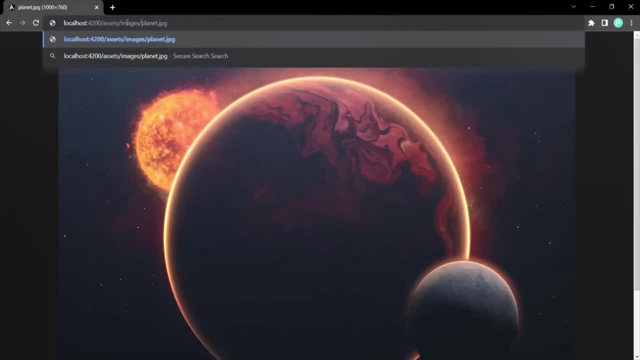 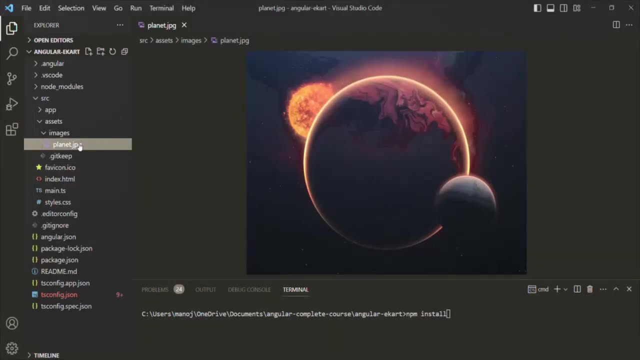 we have images folder and in that images folder we have planetjpg and it is still accessible. but if I go ahead and if I cut this planetjpg from here, so let me just cut it from here and let me put it in some other folder. maybe let me put it inside this app folder itself. 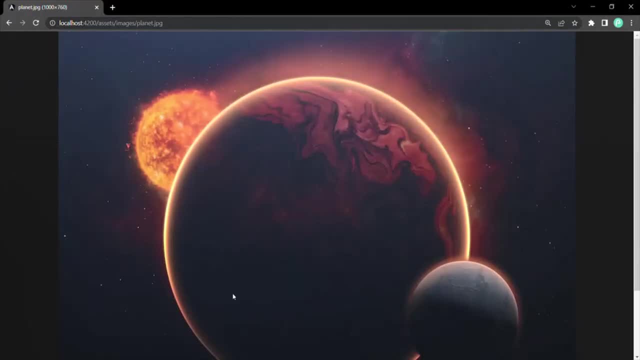 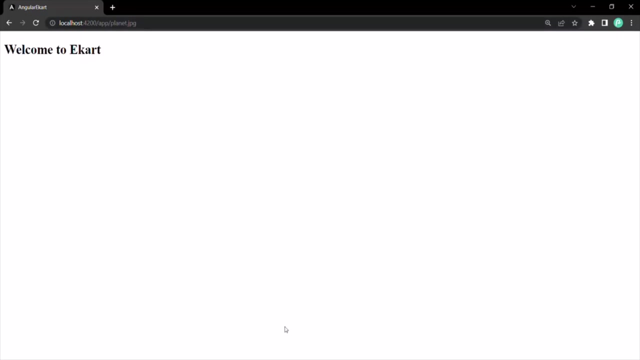 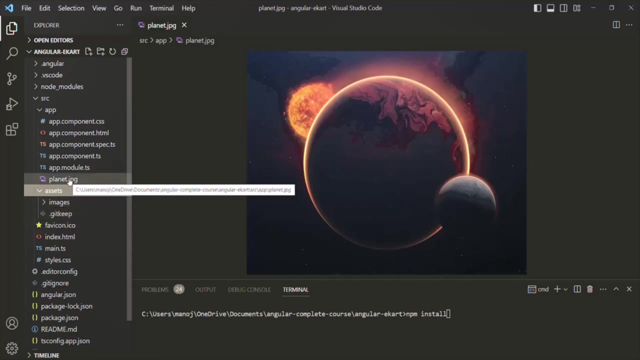 and now, if I go to the browser and if I try to access this planetjpg from that app folder, so if I say app slash planetjpg, if I press enter, you see nothing is rendered here. so only those files and folders which you put inside this assets folder, only that will be accessible publicly. so let me 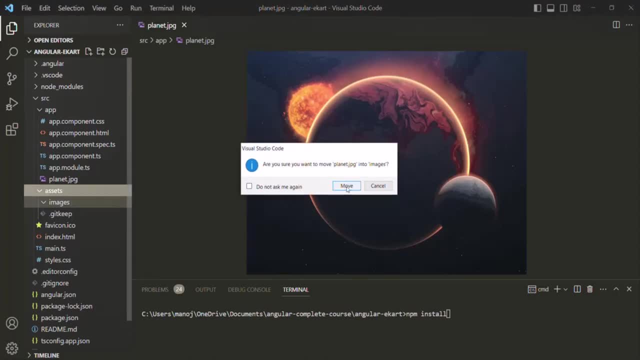 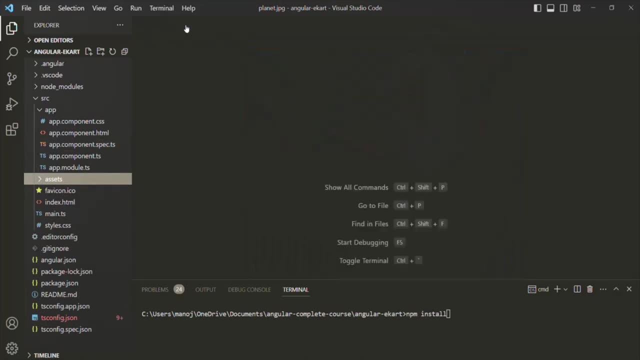 go ahead and let me move it again inside this images folder, all right, so in this folder we keep all our public assets like icons, images, text files, Etc. then we have this faviconico. this is just a simple icon file which will get displayed in the browser. so if I go to the browser, 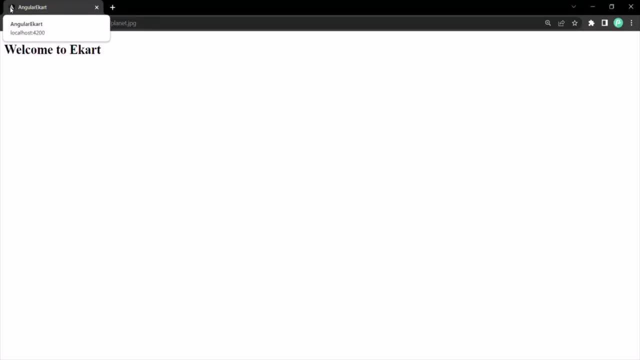 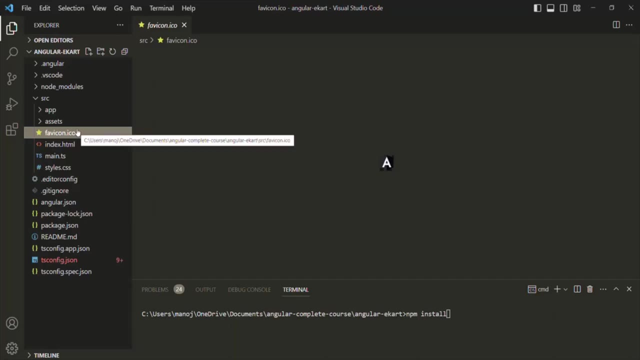 here you will see that favicon has been rendered okay. so, based on your project icon, you can just replace this faviconico with your application favicon. then we have this indexhtml file. this indexhtml file is the Main HTML file which gets rendered in the browser when Angular app runs, and 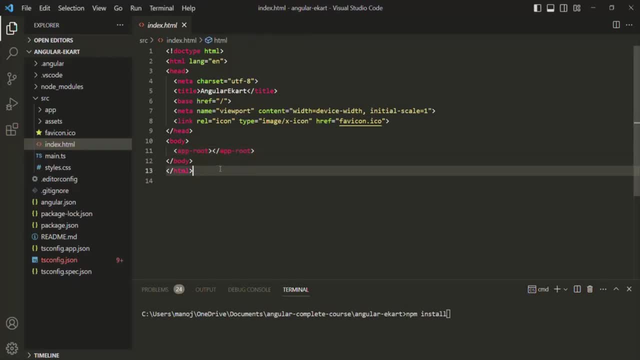 here in this indexhtml file, you will see that we don't have any references to any style sheets or javascript files. this is because all the dependencies will be injected to this indexhtml file during the build process by Angular CLI and we will talk about it more in our coming lectures. 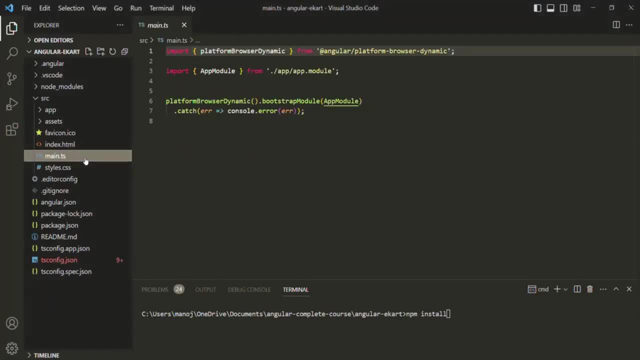 then we have this maints file. so this maints is the TypeScript file and this file is basically the starting point of angular application. so in a lot of programming languages we have this concept of main method, which is the starting point of the application. we have the same concept in angular. 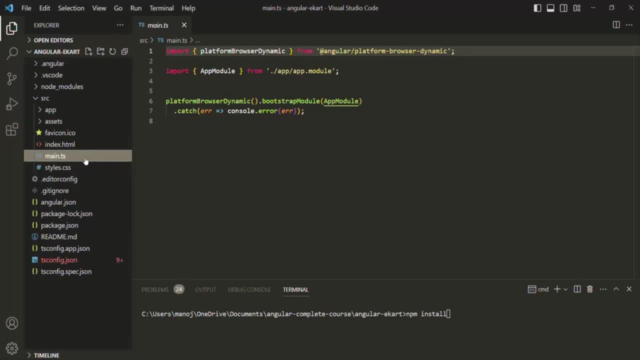 also in this maints file. all we are doing is we are bootstrapping this app module. so when we will run this angular application, it is going to execute this maints file first and there it will load this app module and everything else will start from there. and again we are going to talk more about 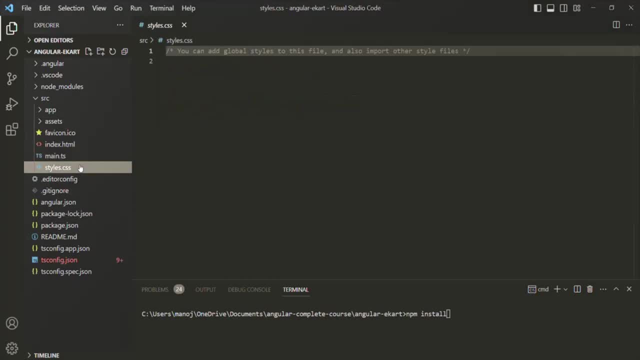 it in our next lecture. then we have this stylecss file. this is where we add all the global CSS styles for our angular application. so whatever CSS style we will specify here, that will be applied to each component and each directive. but for each component also we have a CSS file. we call it componentcss.